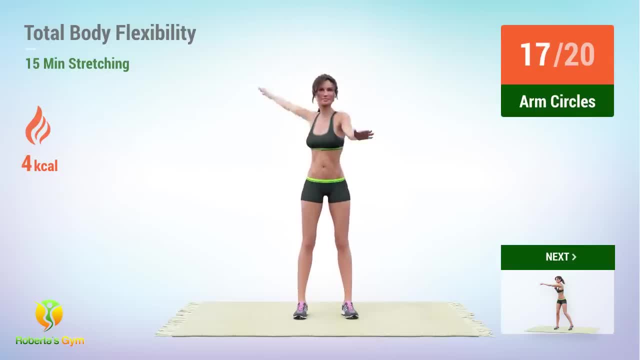 15,, 16,, 17,, 18,, 19,, 20.. Up next punches in: 5,, 4,, 3,, 2,, 1, go 1,, 2,, 3,, 4,, 5,, 6,, 7,, 8,, 9,. 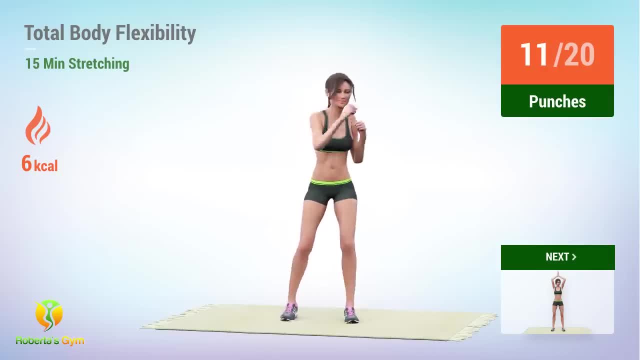 10,, 11,, 12,, 13,, 14,, 15,, 16,, 17,, 18,, 19,, 20.. Up next prayer pushes in 5,, 4,, 3,, 2,, 1, go. 1,, 2,, 3,, 4,, 5,, 6,, 7,, 8,, 9,, 10,, 11,, 12,, 13,, 14,, 15,, 16,, 17,, 18,, 19, 20.. 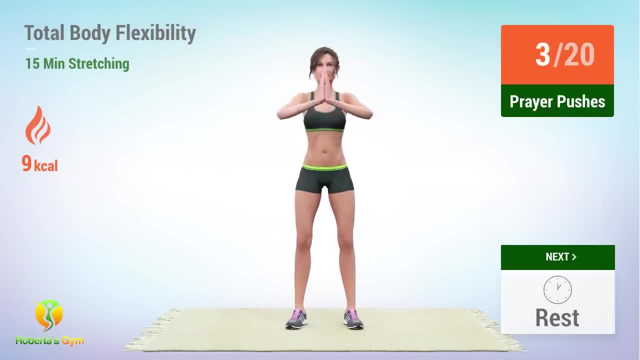 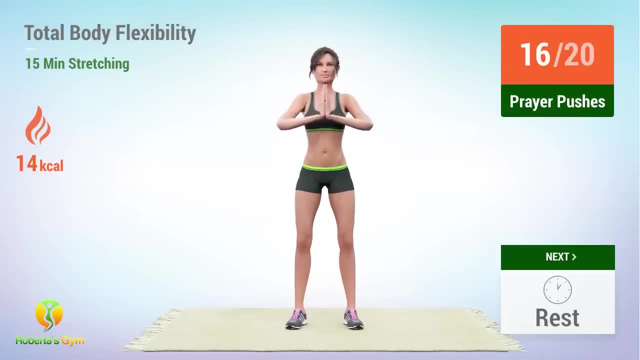 Up. next prayer pushes in: 5,, 4,, 3,, 2,, 1, go 1,, 2,, 3,, 4,, 5,, 6,, 7,, 8,, 9,, 10,, 11,, 12,, 13,, 14,, 15,, 16,, 17,, 18,, 19,, 20.. 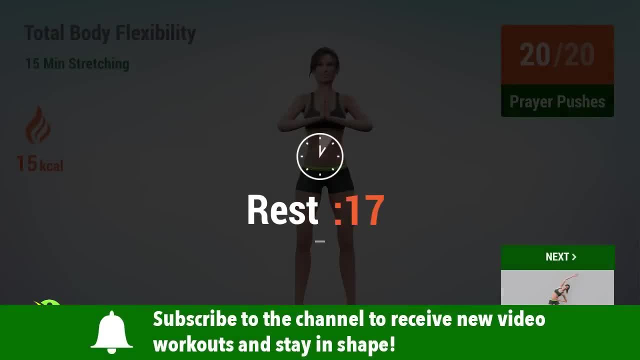 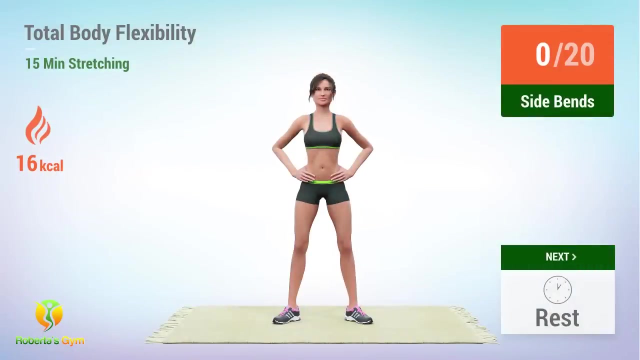 Rest time. Up next side bends In 5,, 4,, 3,, 2, 1, go 1,, 2,, 3,, 4,, 5,, 6,, 7, 8. Congratulations, you've passed the 3 minute mark. 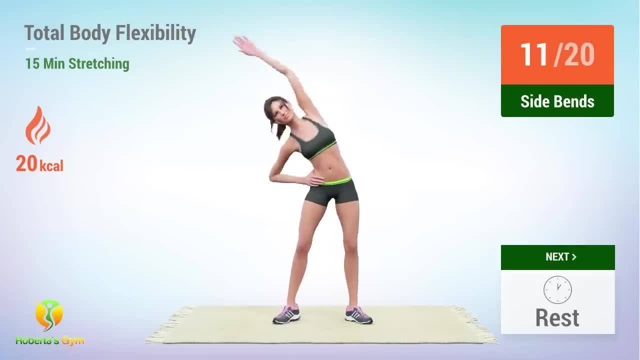 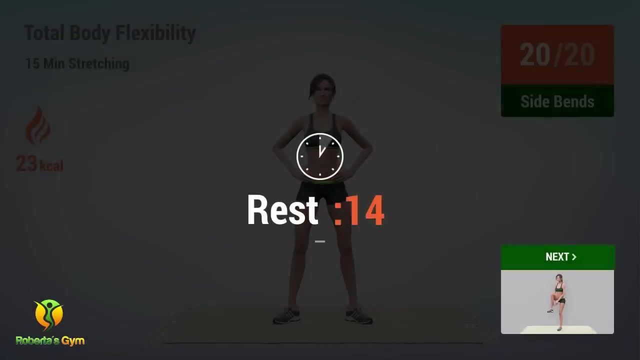 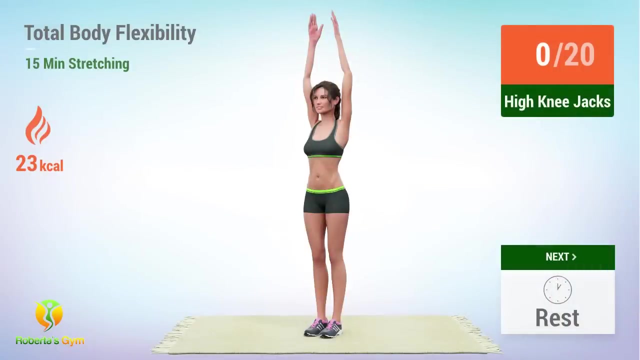 Keep working out. let's see how far you can go. 11,, 12,, 13,, 14,, 15,, 16,, 17,, 18,, 19, 20 Rest time. Up next, high knee jacks In 5,, 4,, 3,, 2,, 1, go. 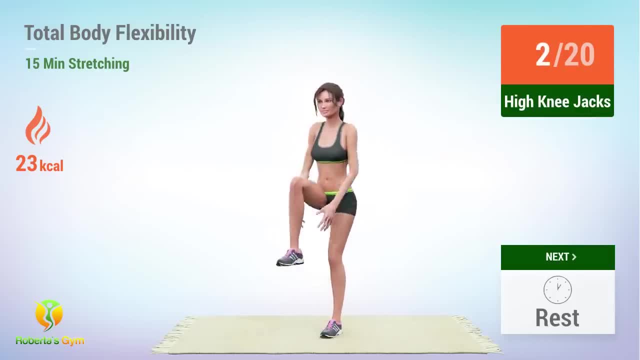 1,, 2,, 3,, 4,, 5,, 6,, 7,, 8, 9,, 10,, 11,, 12,, 13,, 14,, 15,, 16,, 17,, 18,, 19, 20. 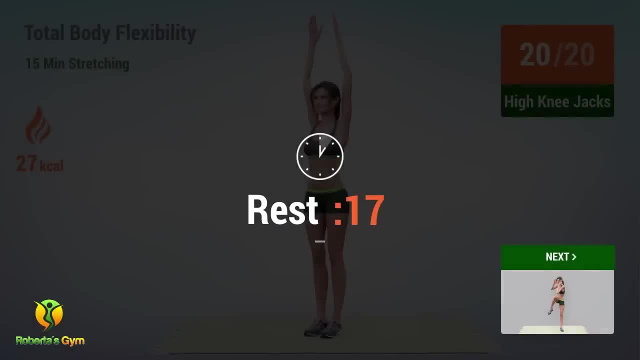 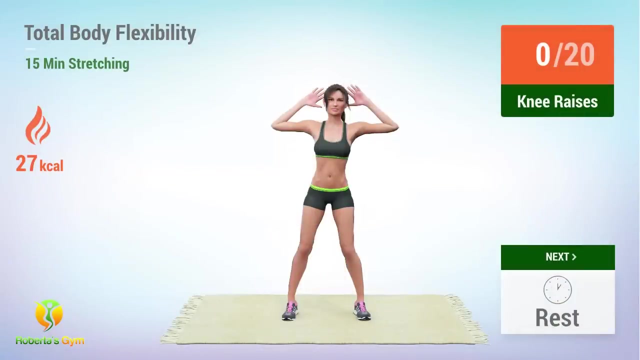 Rest time. Up next knee raises In 5,, 4,, 3,, 2, 1, go 1,, 2,, 3,, 4,, 5,, 6,, 7,, 8, 9,, 10,, 11,, 12,, 13,, 14,, 15,, 16,, 17,, 18,, 19, 20. 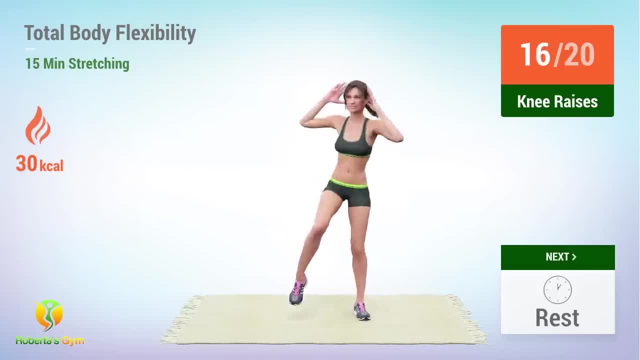 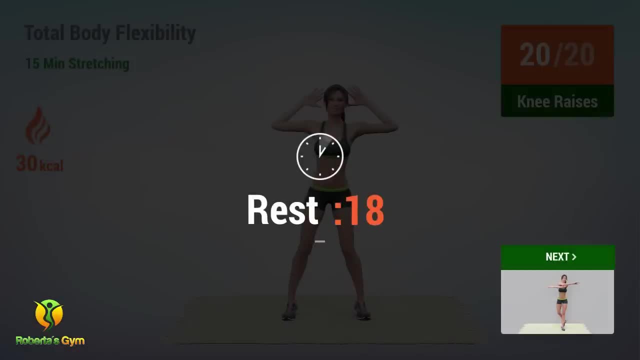 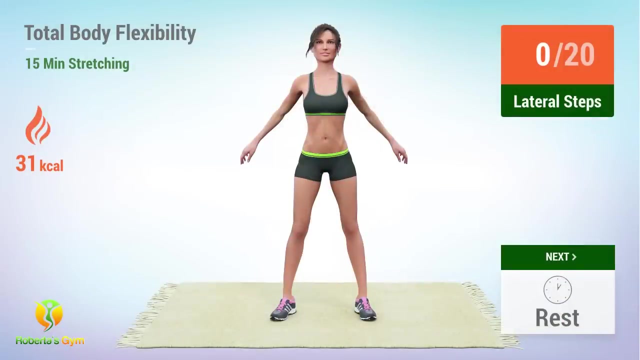 Rest time. Up next high knee jacks In 5,, 4,, 3,, 2,, 1,. go Up next high knee jacks In 5,, 4,, 3,, 2, 1,. go Up next lateral steps. 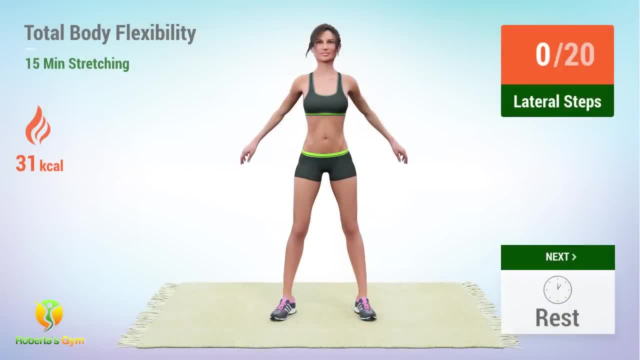 In 5,, 4,, 3,, 2,, 1, go 1,, 2,, 3,, 4,, 5,, 6,, 7,, 8,, 9,, 10,, 11,, 12,, 13,, 14,, 15,, 16,, 17,, 18,, 19, 20. 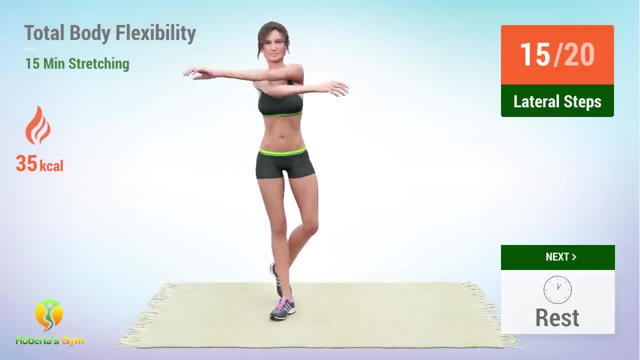 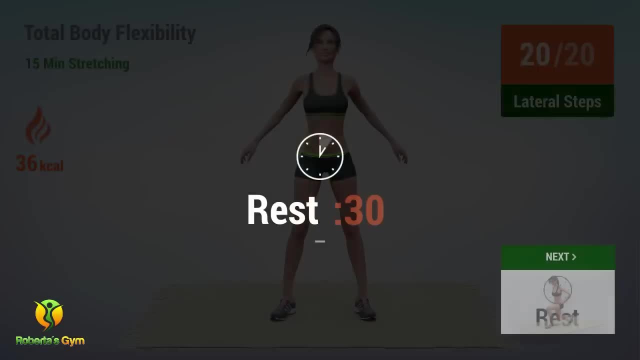 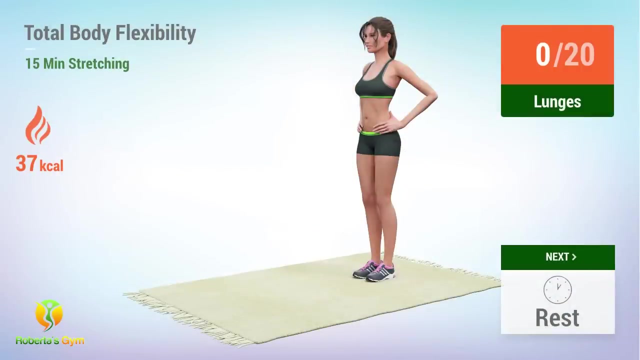 Rest time. Up next high knee jacks In 5,, 4,, 3,, 2,, 1, go. Up next knee raises In 5,, 4,, 3,, 2, 1, go 1,, 2,, 3,, 4,, 5,, 6,, 7,, 8,, 9,, 10,, 11,, 12,, 13,, 14,, 15,, 16,, 17,, 18,, 19,, 20. 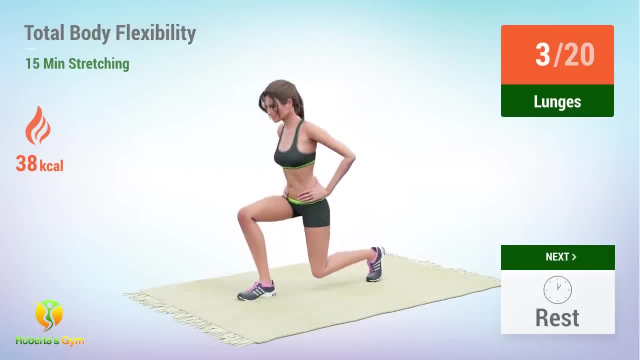 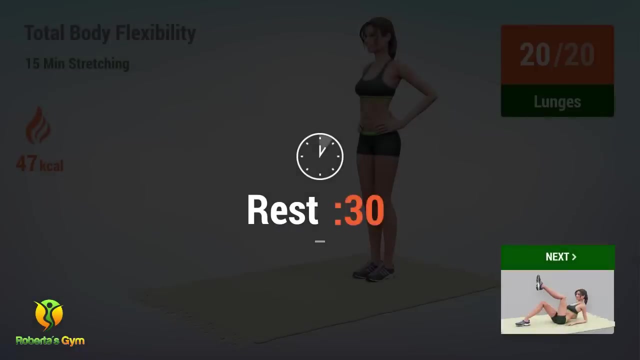 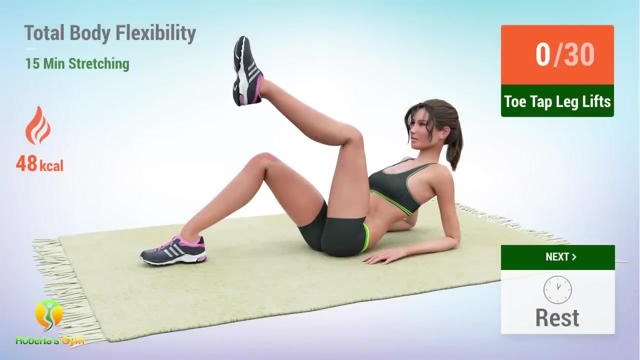 Rest time In 5,, 4,, 3,, 2, 1, go Twelve, Thirteen, Fourteen, Fifteen, Sixteen, Seventeen, Eighteen, Nineteen, Twenty Rest time Up next Toe Tap Leg Lifts In five, four, three, two, one go. 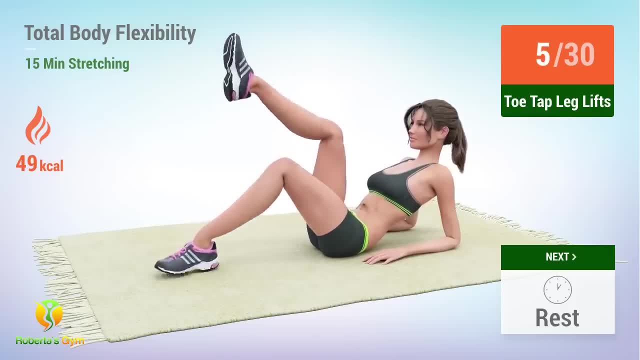 One, two, three, four, five, six, seven, eight nine. ten One, two, three, four, five, six, seven, eight nine. twenty One two, three, four, five, six, seven, eight nine thirty. 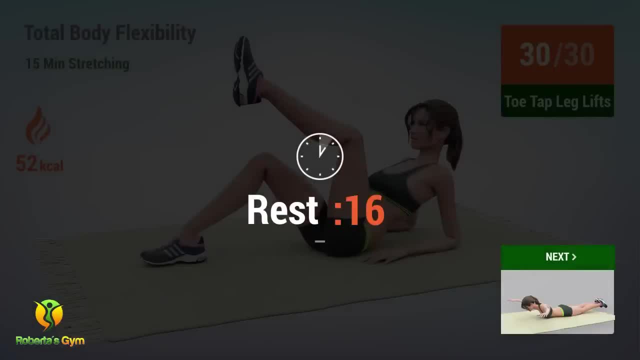 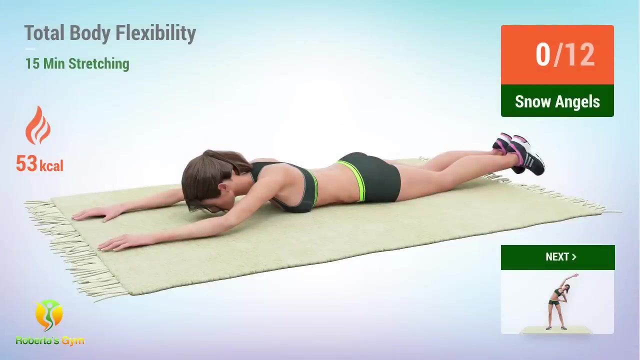 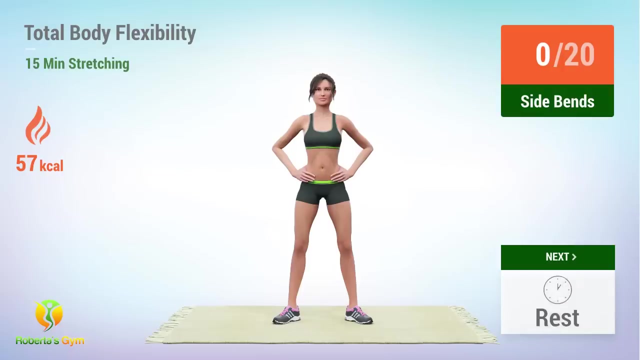 Rest time Up next Snow Angels. In five, four, three, two, one go. One, two, three, four, five, six, seven, eight, nine, ten, Eleven, twelve, Up next Side Bends. In five, four, three, two, one go. 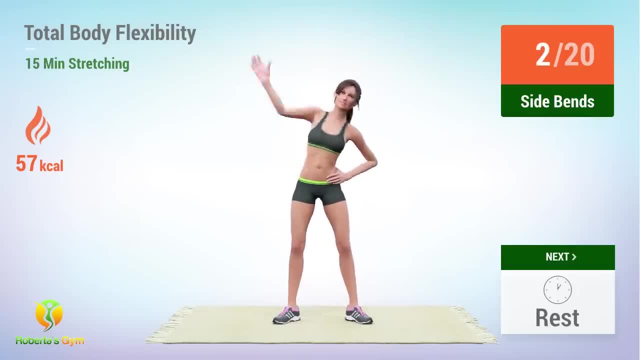 One, two, three, four, five, six, seven, eight, nine, ten, Eleven, twelve, Thirteen, Fourteen, Fifteen, Sixteen, Seventeen, Eighteen, Nineteen, Twenty Rest time Up next Toe Tap Leg. Lifts In five, four, three, two, one go. 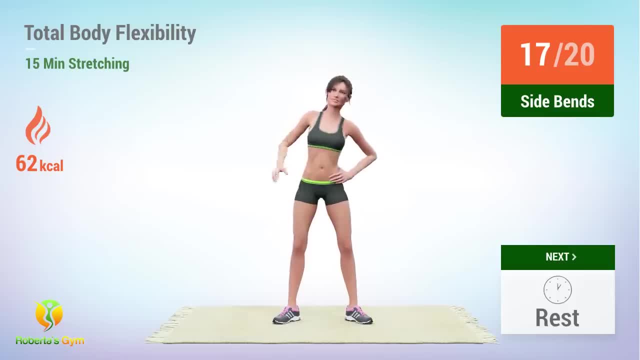 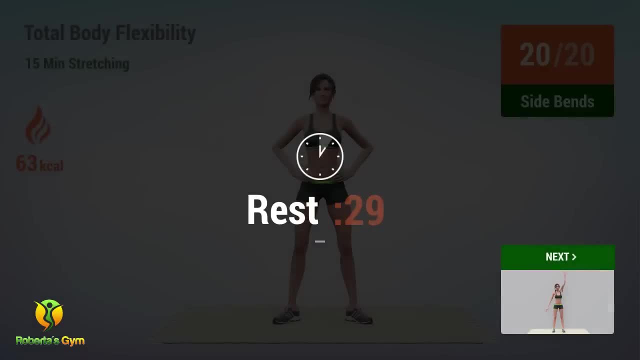 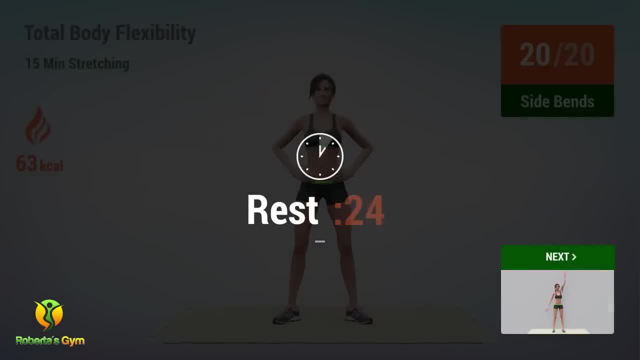 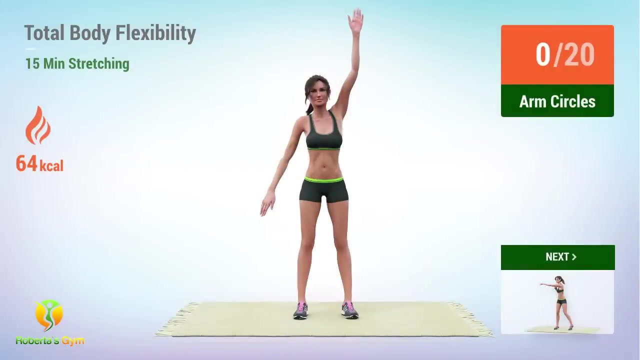 Thirteen Up next arm circles In 5,, 4,, 3,, 2,, 1, go 1,, 2,, 3,, 4,, 5,, 6,, 7,, 8,, 9,, 10,, 11,, 12,, 13,, 14,, 15,, 16,, 17,, 18,, 19, 20.. 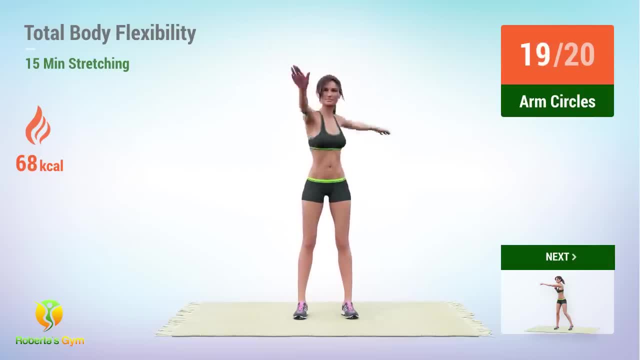 Up next punches In 5,, 4,, 3,, 2,, 1, go 1,, 2,, 3,, 4,, 5,, 6,, 7,, 8,, 9,, 10,, 11,, 12,, 13,, 14,, 15,, 16,, 17,, 18,, 19,, 20.. 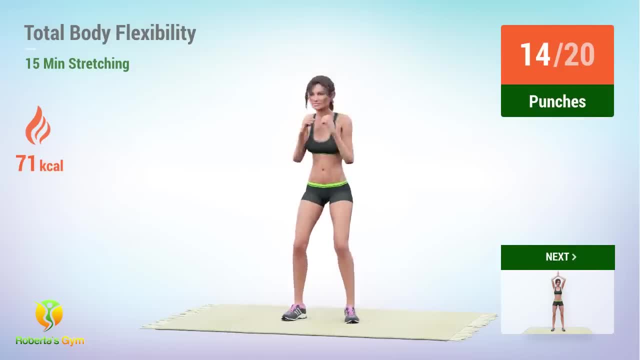 Up next prayer pushes: 1,, 2,, 3,, 4,, 5,, 6,, 7,, 8,, 9,, 10,, 11,, 12,, 13,, 14,, 15,, 16,, 17,, 18,, 19,, 20..